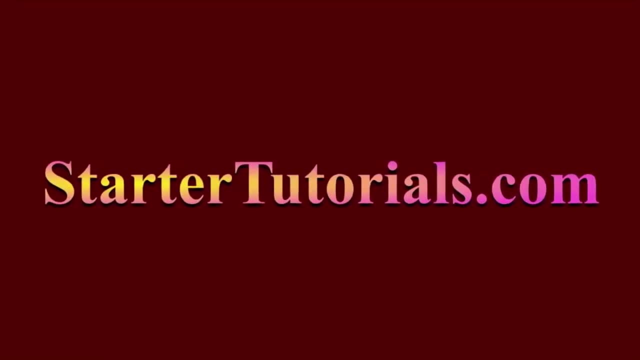 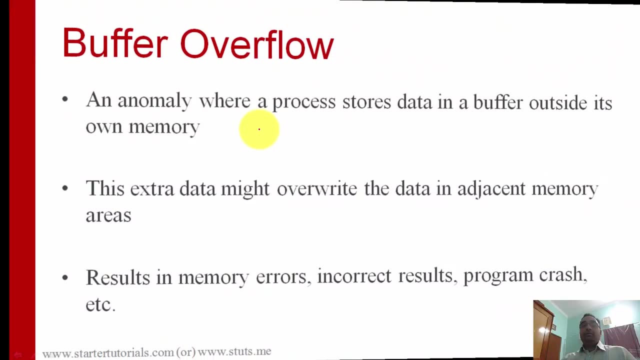 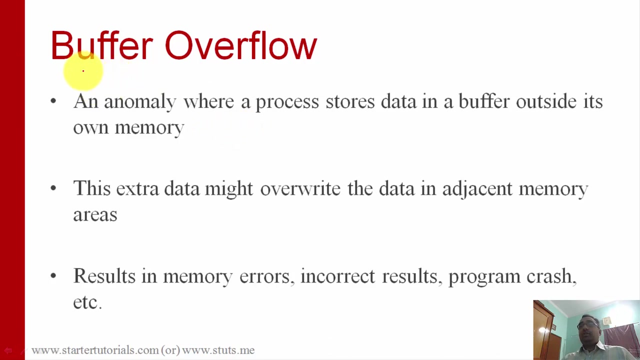 Hello everyone, welcome to the session on cyber security. So in this session we are going to look at another technique called Buffer Wawapo. Okay, so this is also a technique related to the logic of the application. So in Buffer Wawapo it is dependent on a vulnerability. 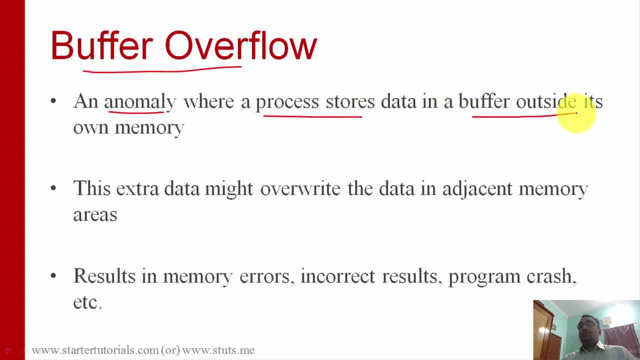 where the process stores data in a buffer outside its own memory. Okay, so you can consider buffer as an array and it is normal in programs to store data in arrays or buffers, And whenever you are using arrays or buffers in a program in languages like C, where there is no bounds, 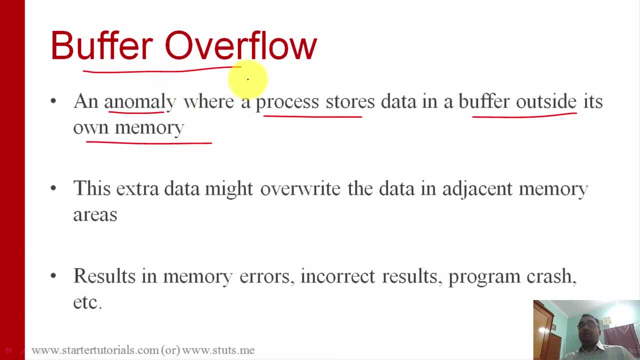 checking. you should be careful, Otherwise Buffer Wawapo attacks can be possible. Okay, so in this attack the attacker will provide extra data while giving input or in some other way they will give extra data that is malicious data, which will override the data in adjacent. 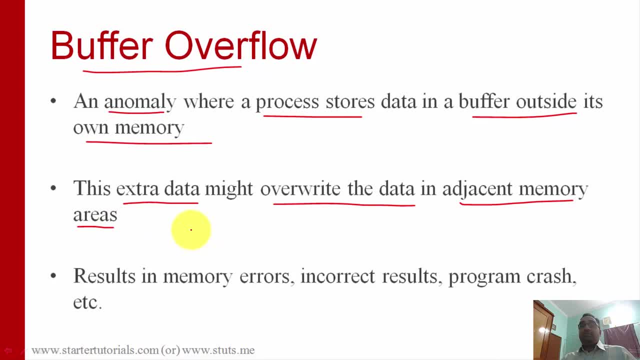 memory areas- In the next coming few slides we will see an example of this- memory locations etc. And when giving such extra data, which will override adjacent memory locations, that will result in memory errors, incorrect results as well as program crash. Okay, so which is? 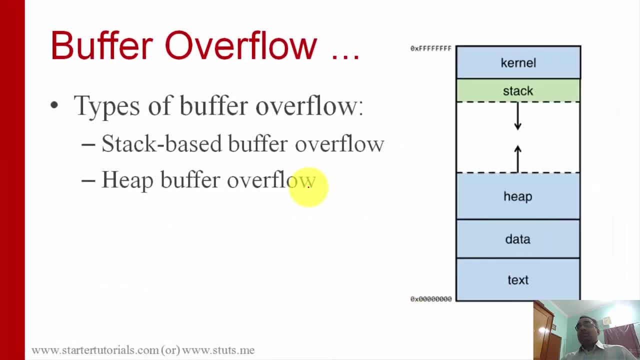 like a denial of service attack. So there are two types. One is stack based buffer power flow and heap based buffer power flow. So this is the process image for every process running on your system In the random access memory. that is the stamp, the process image. 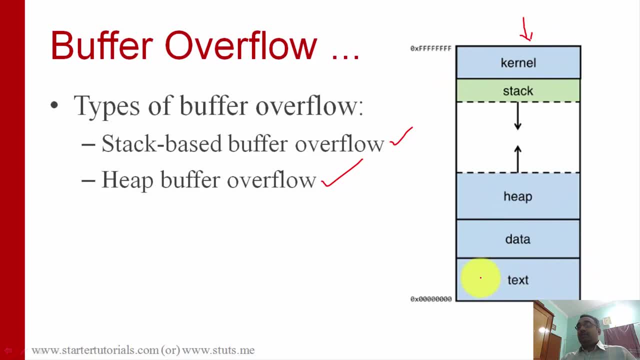 will be created. Okay, so every process will have text segment, data segment, heap area where data will be stored, runtime data, and you will have a stack where functions will be stored, And on top of that you have a kernel which belongs to the operating system. 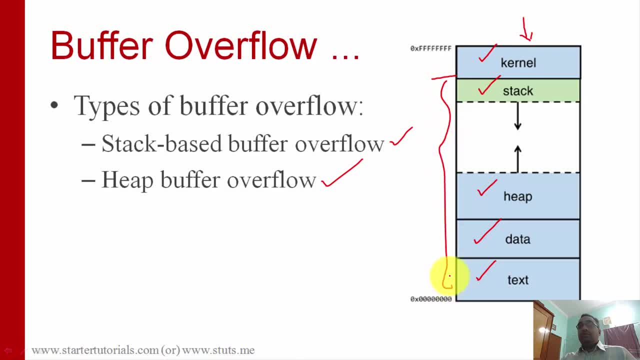 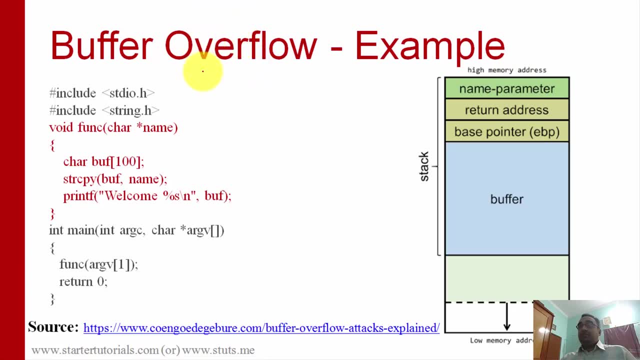 So this is the process image from here to here. Okay, So let's consider an example for buffer power flow, And this is for stack based buffer power flow. Consider this C code program, which is written in C. So here is a function called func, which is accepting a parameter. So it is basically. 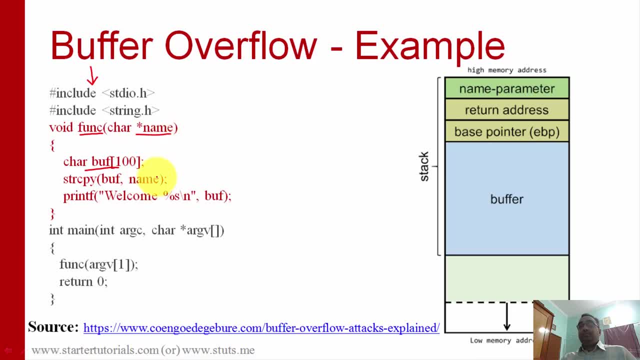 a string pointer to a string where I will give the data here. Okay, So this will go to the parameter name And inside the function we are getting a character array which is named buff. So this is our buffer of size 100.. 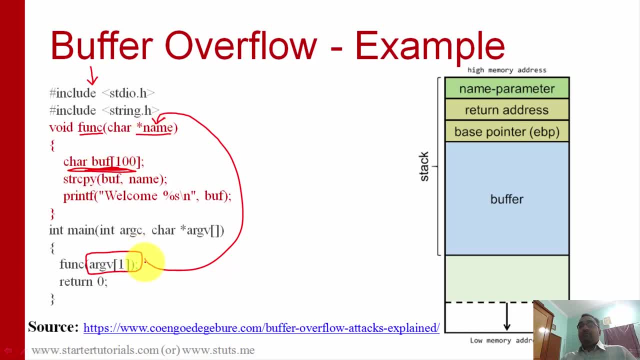 And inside the function we are getting a character array which is named buff. So this is our buffer of size 100.. And whatever data I am giving here, I am popping it into buffer. Okay, buffer array. And finally, 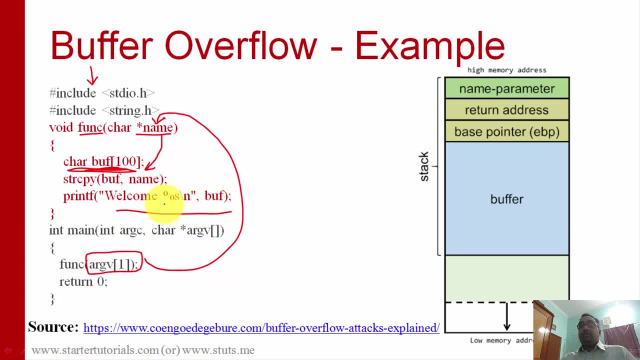 I am printing that data. For example, if I do ramesh here, it will print welcome ramesh. So this is a simple program. looks simple, Okay. So how can this program be used for performing buffer power flow is? before going to that, let's look at the process image. 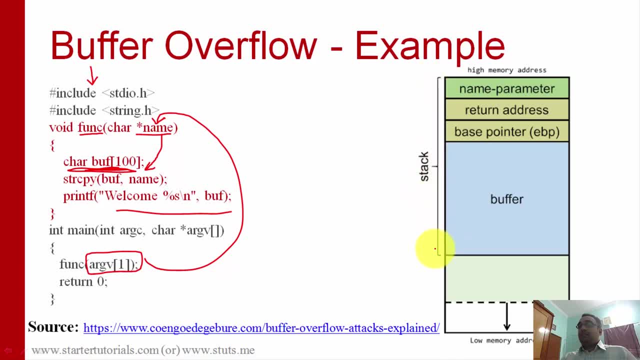 You can see on the right hand side. So here is the stack from here to here. You can think of the bottom locations. like you have heap text segment, data segment, don't worry about that. So consider the stack. So here, this memory is for name, Okay, And this is the. 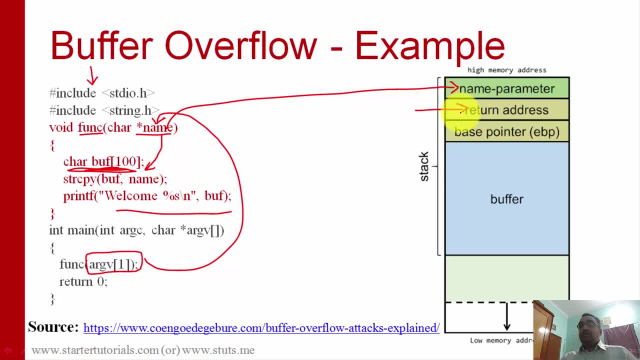 return address function: return address. So the function is called here, So the address of this location will be stored here, And this is a base pointer which is related to the function. And here is the buffer array. So, from here to here, this is your buffer. 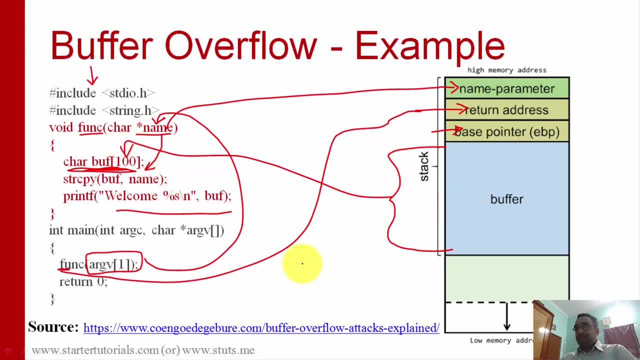 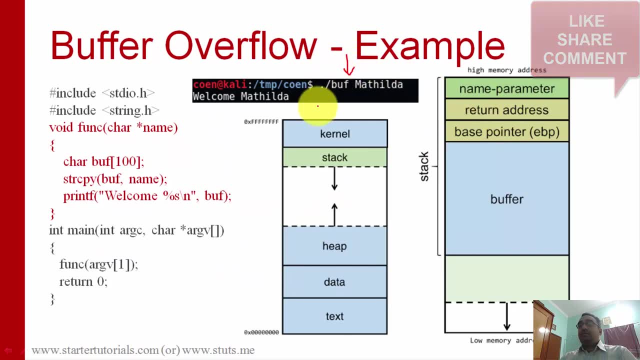 array. Okay, Now see here. So when it is when the program is executed, normally, you will execute like this. So I think this is Linux or Unix based system. So we will run the C programs like this: dot slash program name followed by the data. So this data goes into here And 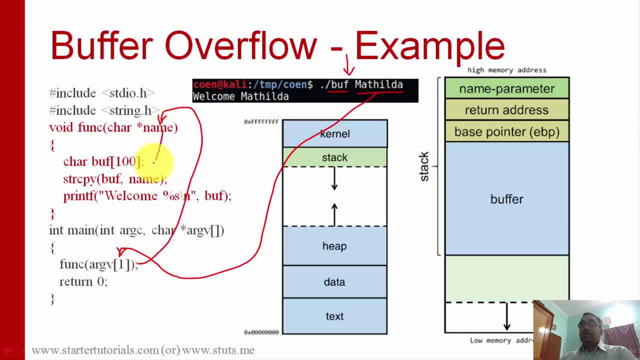 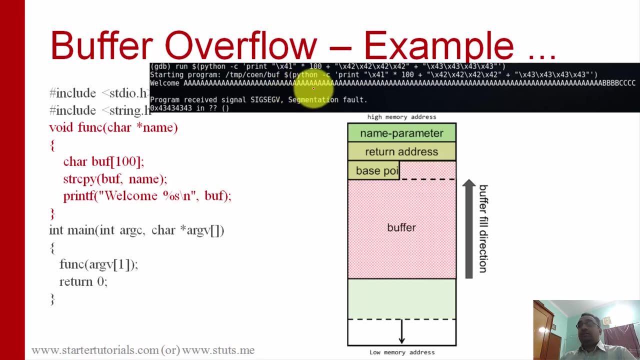 from here it goes into name, And from name it is stored into buffer array. So that's it, Okay, And the output is this: welcome Matilda. Now see here, instead of giving text like Matilda, et cetera, they are giving code like this: Okay, So by using this code, what will? 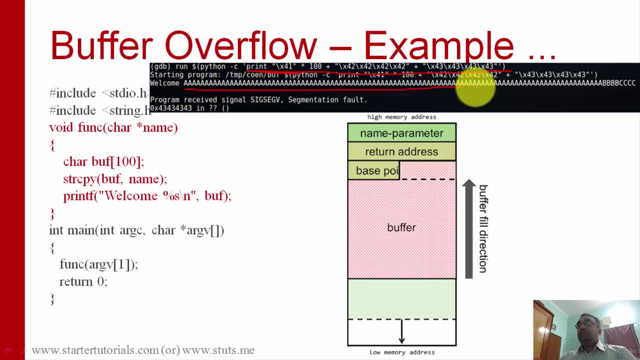 happen is: this will be given as input. Okay, And if the data is given in multiple arrays, what we are going to need to do is, in order to get the maximum number of runs we are going to need to, what we are going to do is: 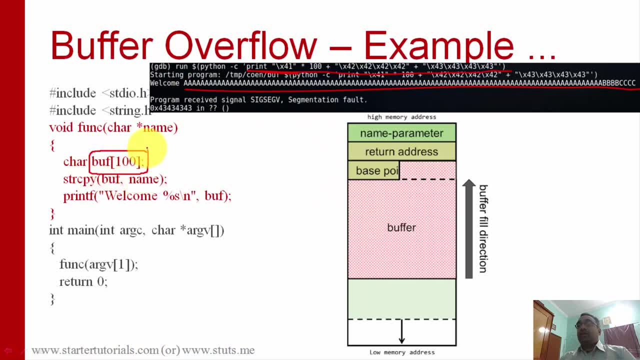 we are going to use a multicolor array. So we are going to use the multicolor array and that will be 1, 1, 1, 1, 1, 1, 1.. 4 B's and 4 C's: Now what happens? So, actually, this is the size of buffer. Now, since you are 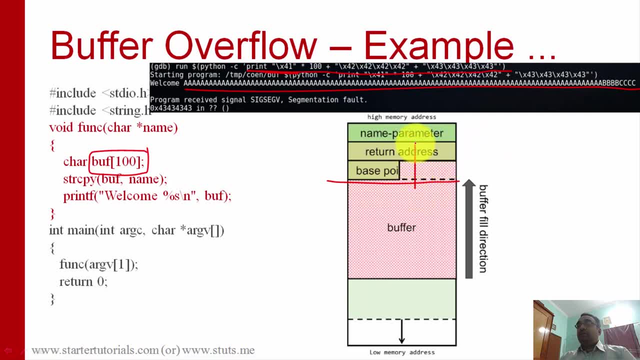 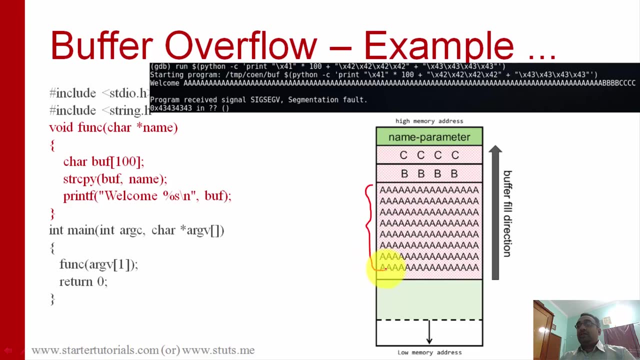 giving BBB CCC also extra data, it will start overwriting this data, Okay. So that's why you can see here: base pointer address location is being overwritten, Okay, And it will be stored like this. So these are the 100 characters: AAA, 4 B's and 4 C's. So your base pointer address.